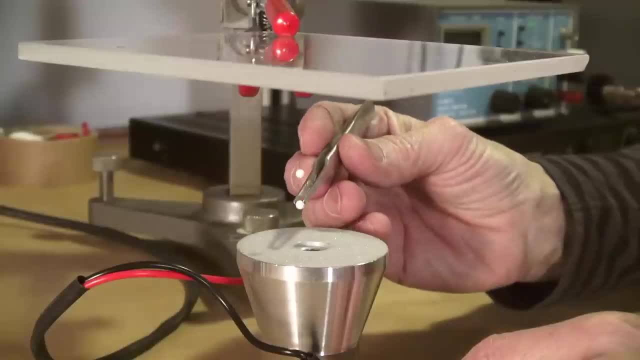 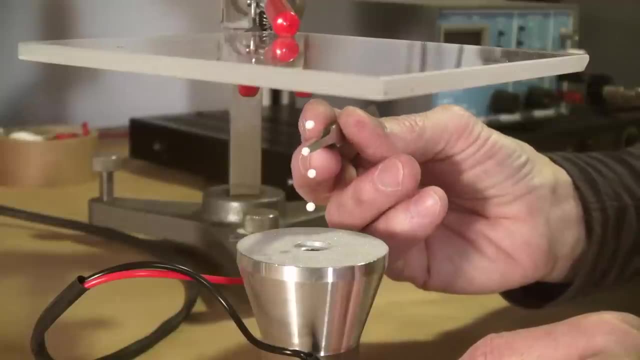 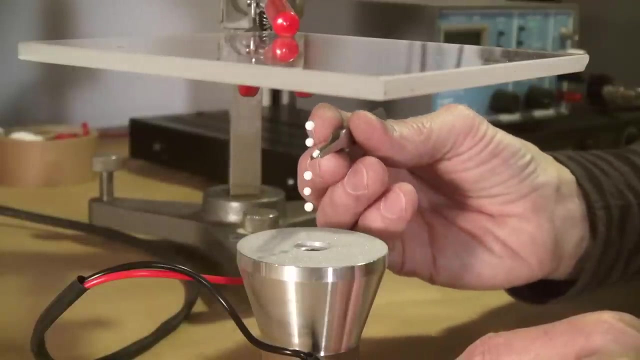 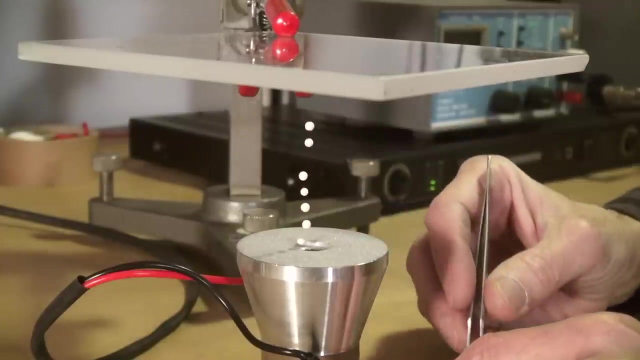 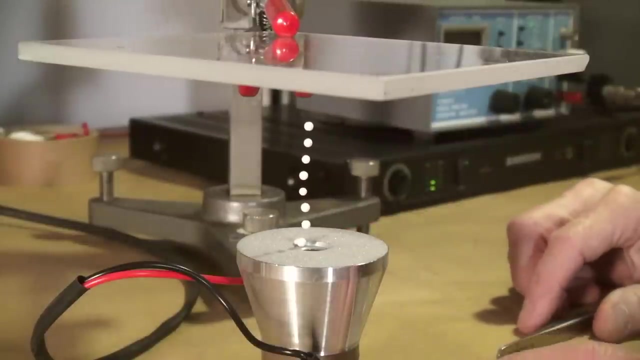 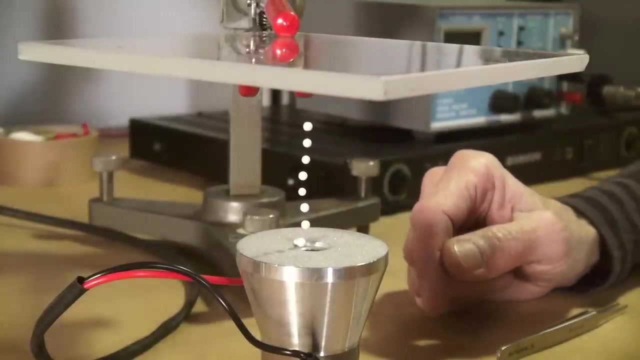 I'm going to go to the speaker. As I said before, the distance between the reflector and the loudspeaker is just right. If I change it, which I'm going to do, you'll see that this standing wave disappears, and 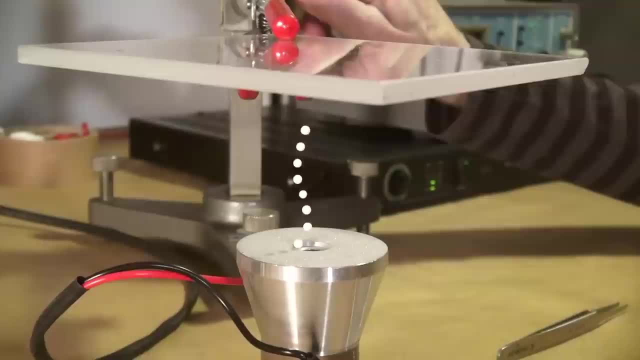 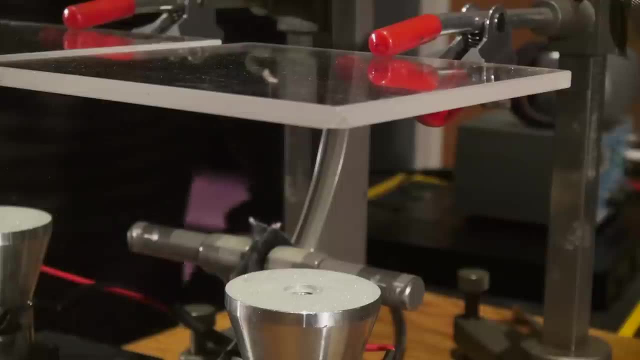 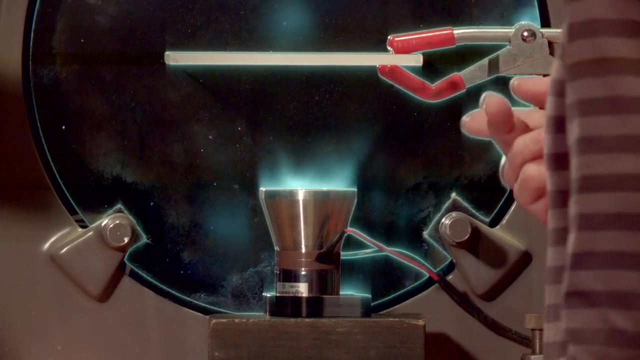 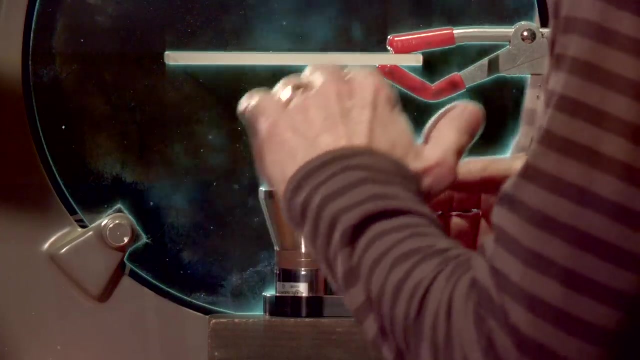 the balls are no longer suspended there. We've now set up the little loudspeaker and the reflector in front of this mirror, which is part of our Schlieren optic setup. The purpose of that is to be able to actually see where there are regions of high pressure. 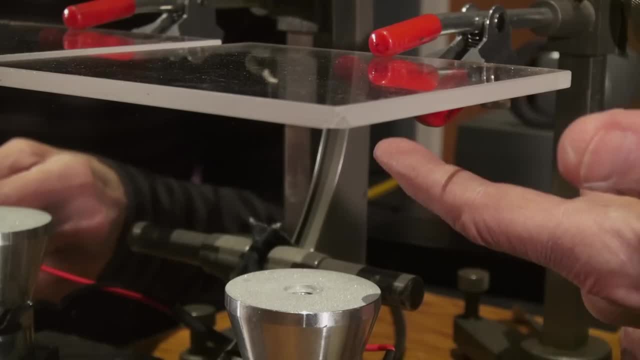 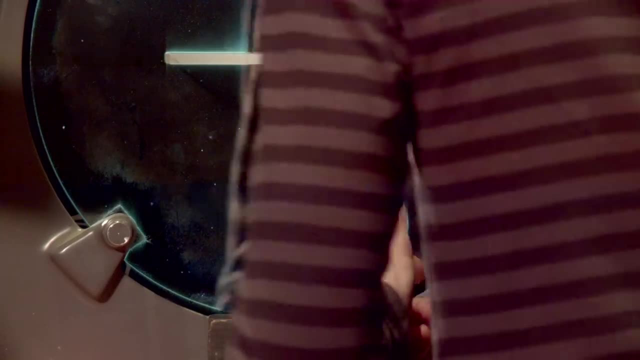 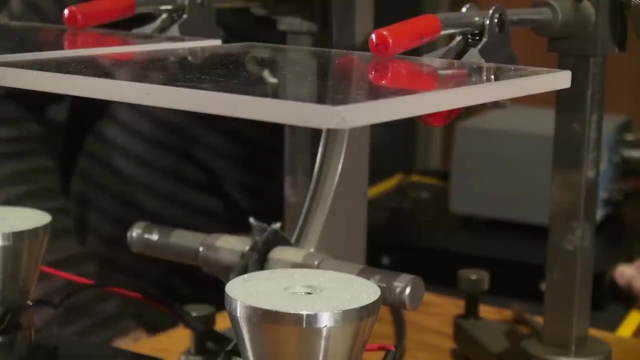 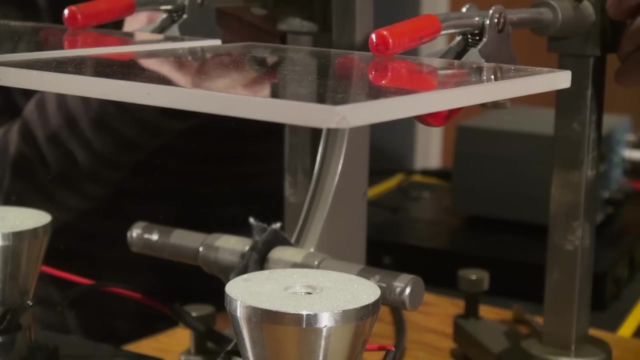 and low pressure in the air, especially the air between the reflector and the loudspeaker. Let me turn up the volume. Before I do that, I will put on my protective hearing, Okay, And if I adjust the height of the reflector, there's a point at which you see bands of 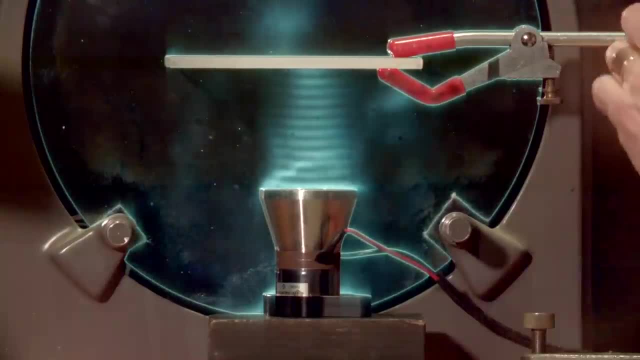 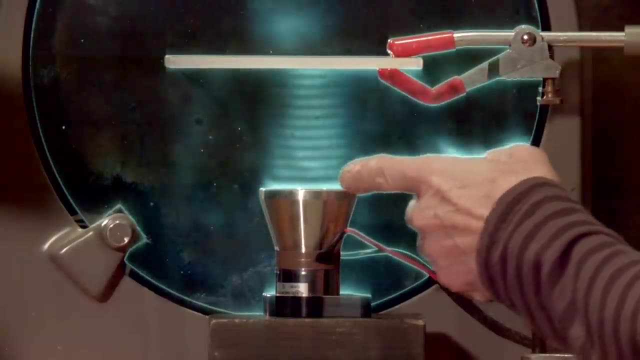 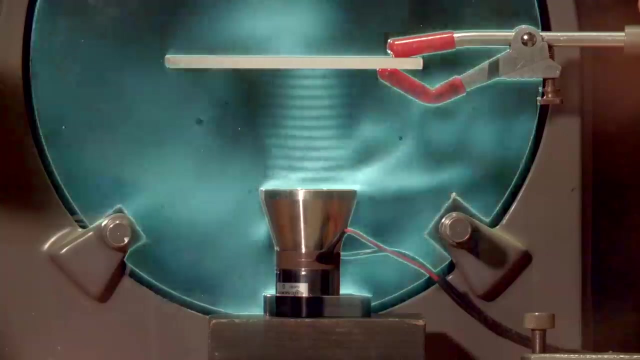 white, light and dark. This is the standing wave, and it only happens when the distance between the reflector and the speaker is some multiple of a half a wavelength. So every standing wave is a half a wavelength. Every single one of those bands is a half a wavelength. 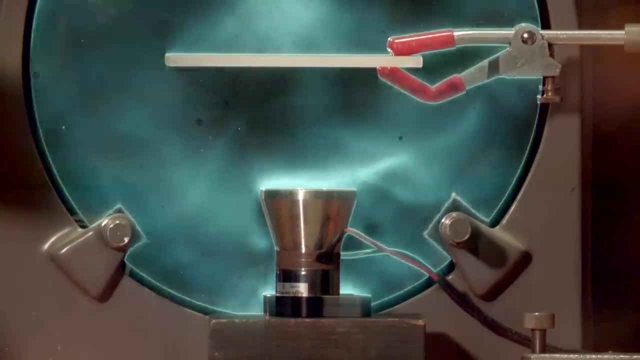 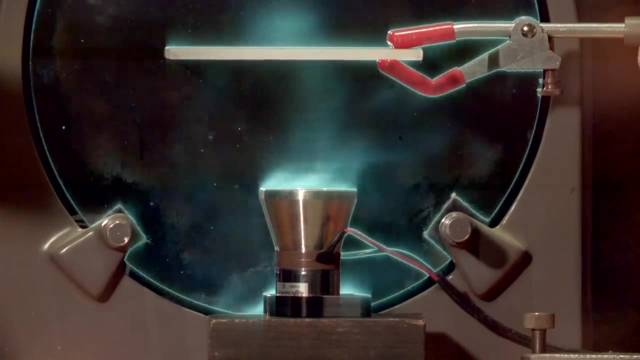 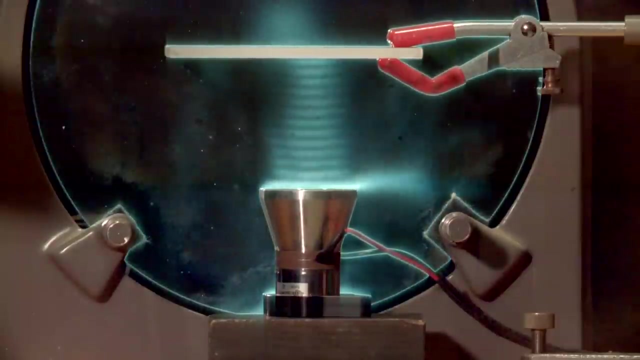 If I go up a little higher, then it disappears again. but if I continue to go higher, then it will come back when I'm at another half a wavelength, a multiple of a half a wavelength, away. Now it's in these bands that I'm going to place the little balls.